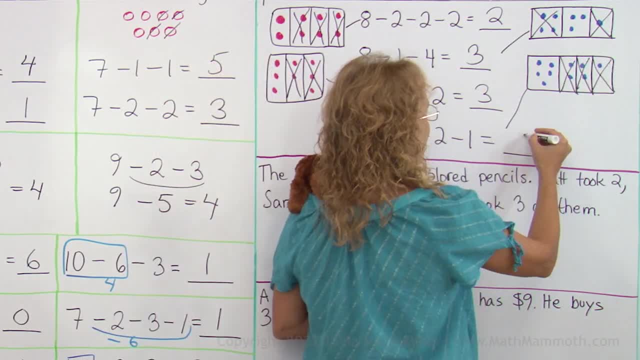 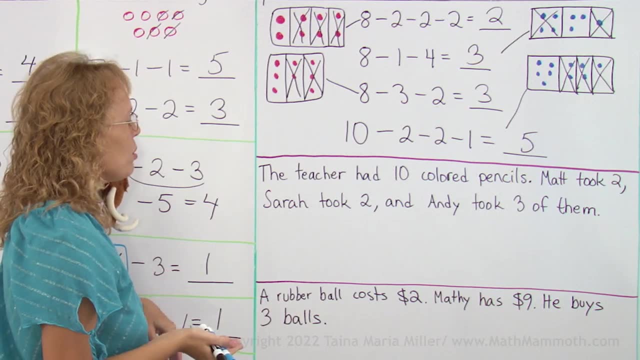 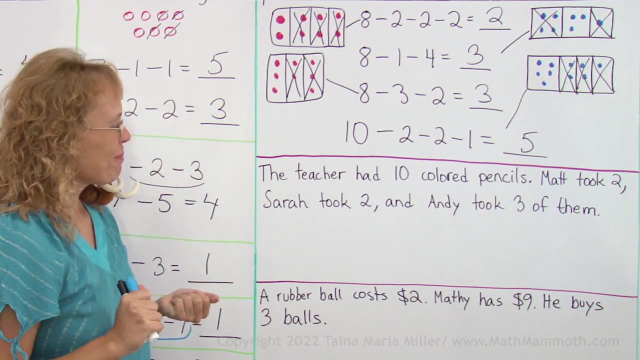 Then minus two, minus two, minus one, and five are left. The teacher had ten colored pencils. Matt took two, Sarah took two and Andy took three of them. What can we ask? I mean it doesn't have any question, right? 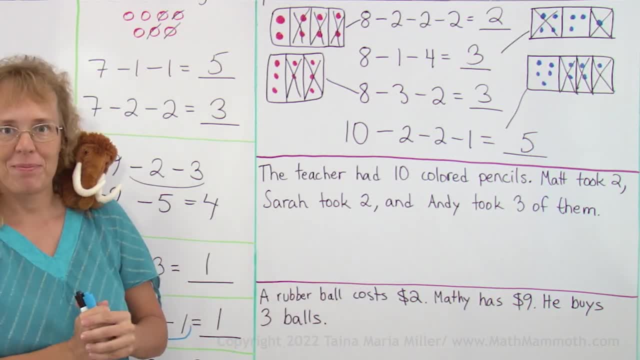 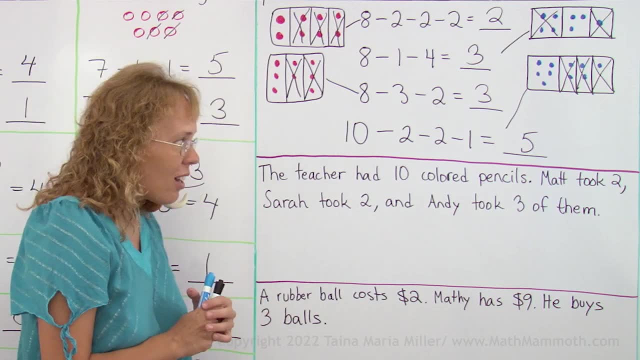 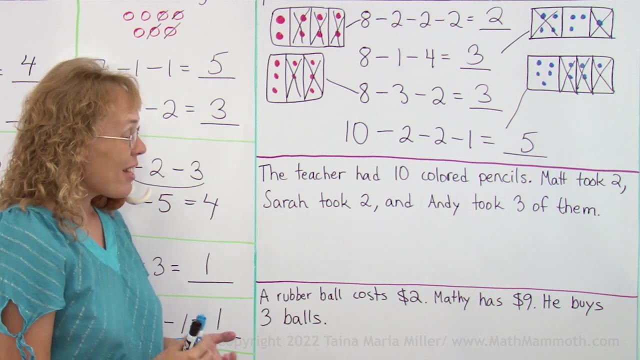 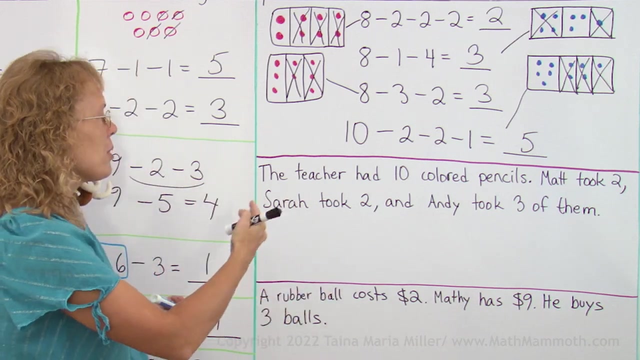 What kind of question can we ask about this situation? Any ideas, Matthew? Matthew's idea is: what colors were the pencils that Andy took? Matthew, you need to make a math word problem. okay, We could ask. okay, there were ten, and Matt took some, Sarah took some, Andy took some. 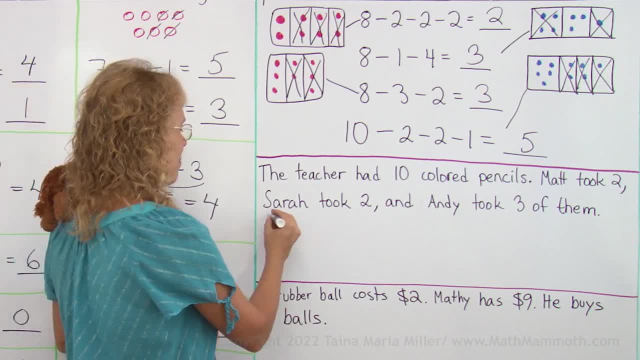 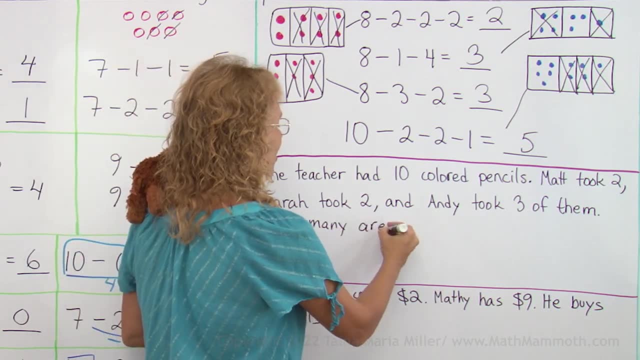 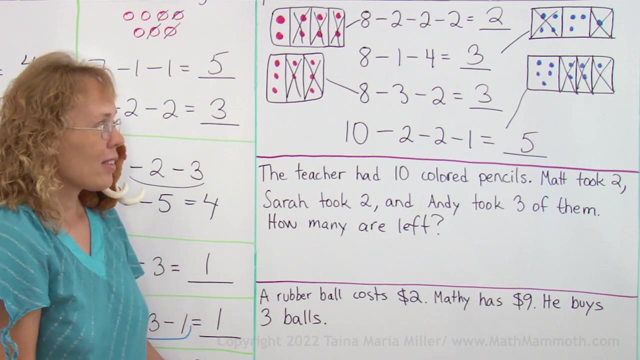 We could ask how many are left right? How many? That's always a good question for a math word problem. How many are left? And now shall we write an addition or subtraction, Or both. You could write a subtraction right. 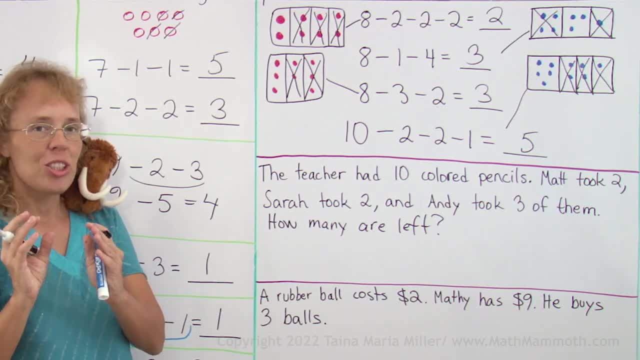 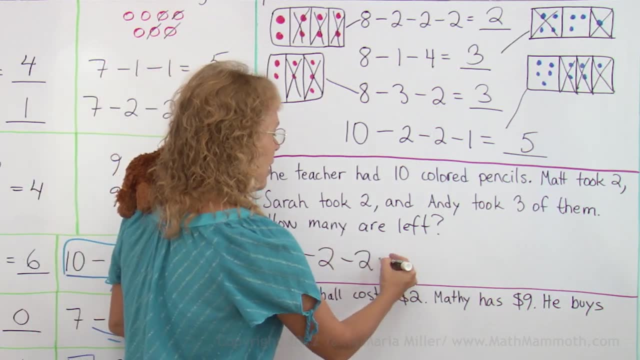 Because there's pencils and some of them go away Or some. you know, these students come and take some. There's ten at first, then two of them are taken, another two are taken and another three are taken. Okay, But to solve it we can think of addition first. 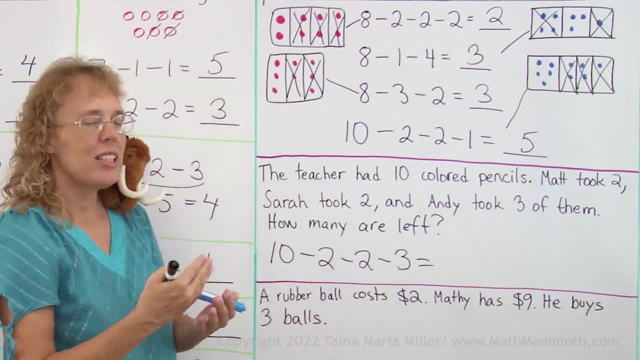 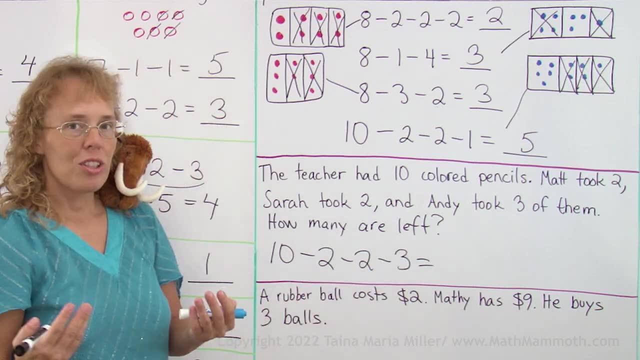 We can add three and two and two. You know how many did they actually take in total? Because two and two makes four plus three, that's seven. So they took a total of seven pencils. Ten minus seven equals three, That's three pencils left. 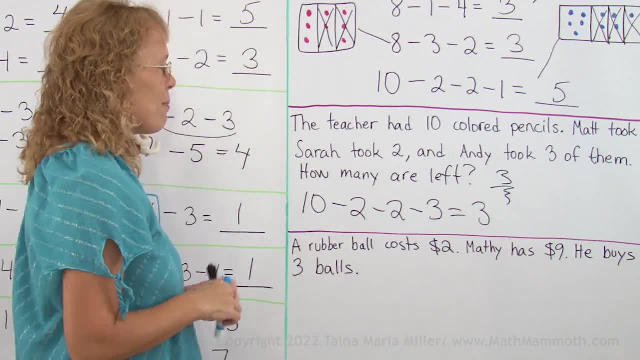 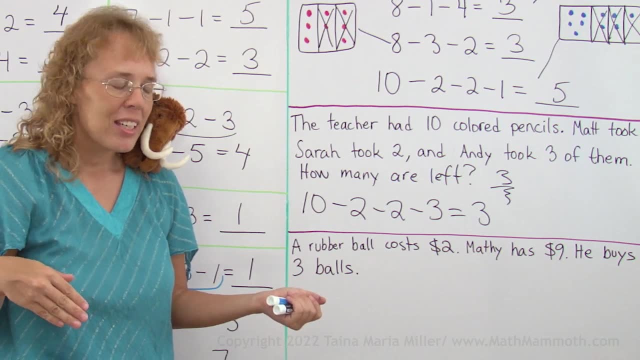 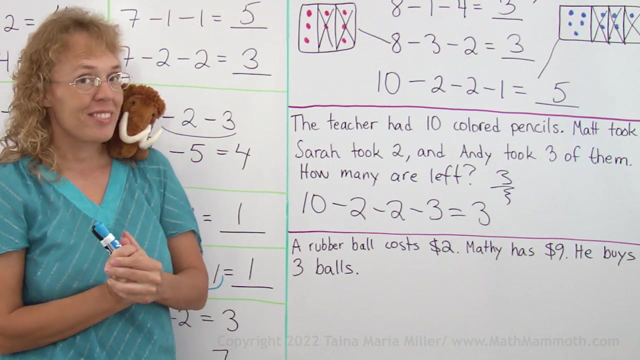 And then, lastly, a rubber ball costs two dollars And Matthew has nine dollars, So he buys three balls. What can we ask? What kind of question can we ask? We can ask. well, one thing we can ask is: how much do those three rubber balls cost? 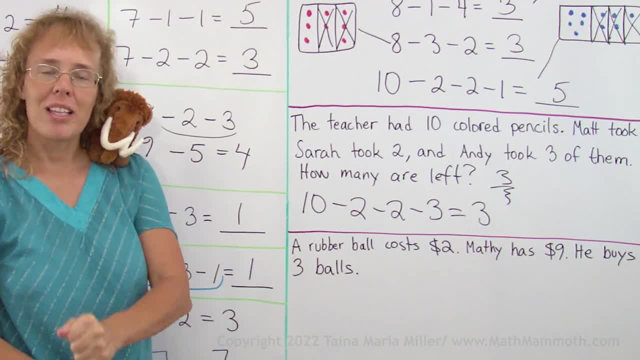 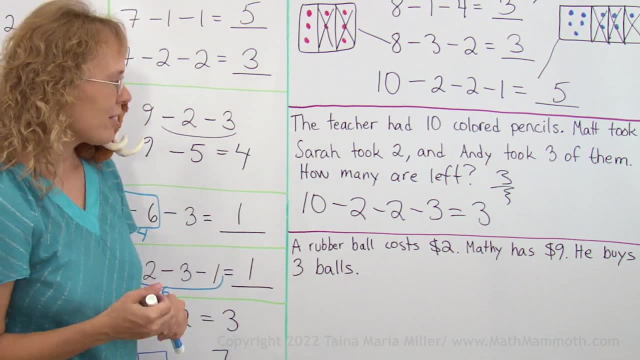 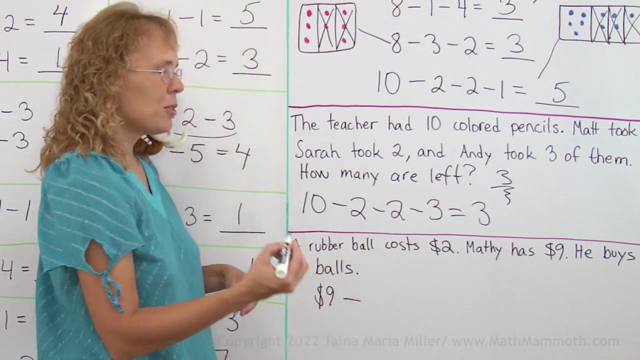 Another thing we could ask is: how much money will Matthew have left after he buys those balls? So let's say we solve how much money Matthew will have left. Matthew would have nine dollars And then he buys, So money goes away from him, right?